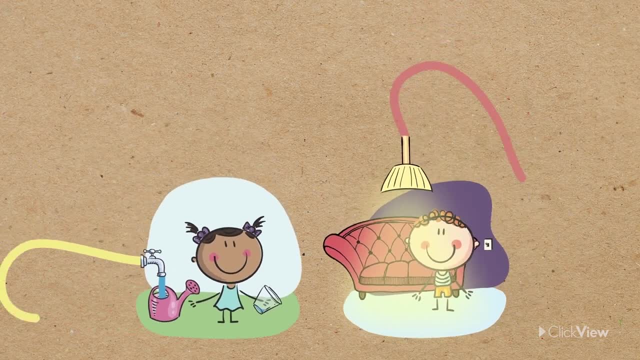 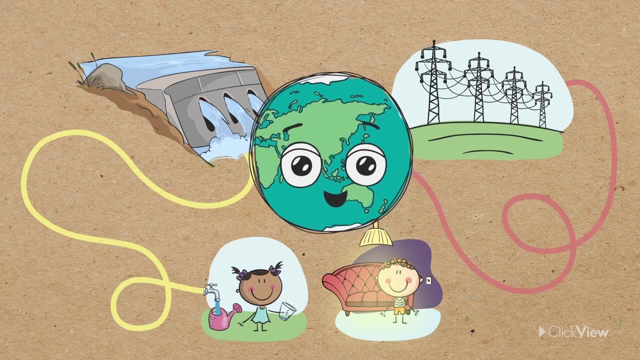 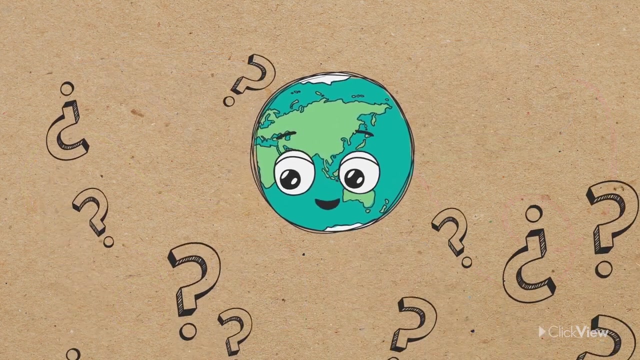 the entire room lights up, But resources don't appear out of thin air. They all come from somewhere and when we don't use them properly, they disappear. That's why we use resources. There can be serious consequences for our world. What can we do to make sure we're using our 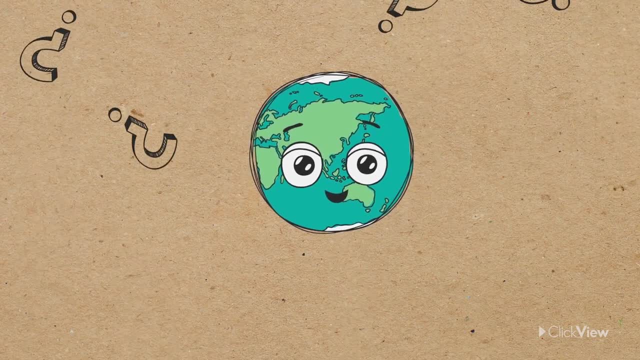 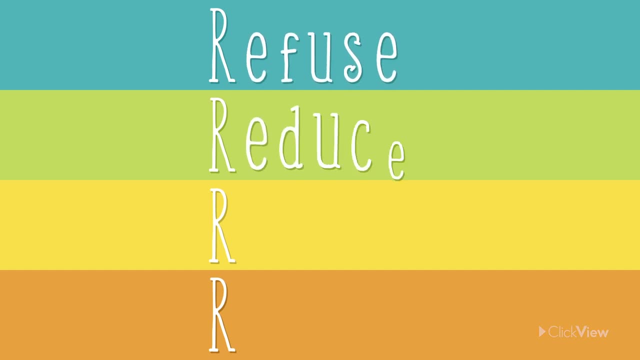 resources thoughtfully Introducing the four R's. The four R's stand for refuse, reduce, reuse and recycle. If everyone follows the four R's together, we can work to use our resources sensibly and keep our planet healthy. What does each R mean? 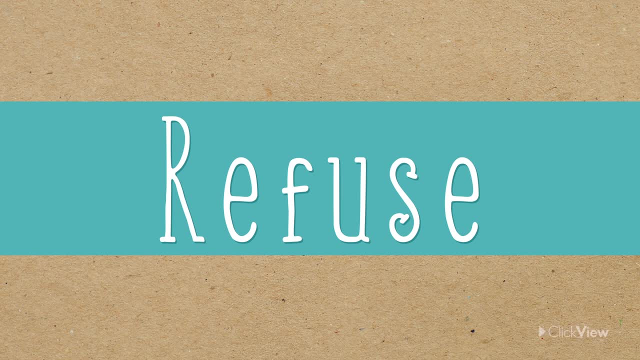 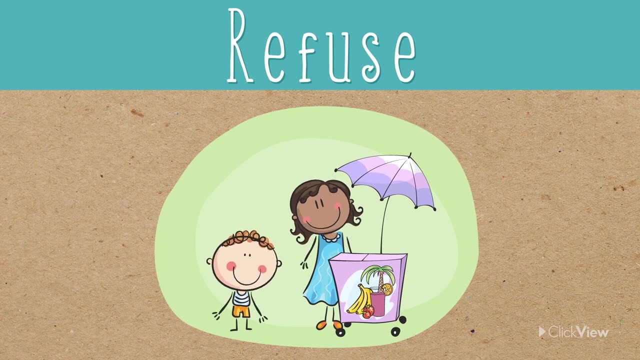 Refuse means saying no to things we don't need. When you're about to use something that you're probably going to throw away straight after, like a plastic straw, think: do I really need to use this? If the answer is no, then say no thanks. Instead, you could drink your smoothie. 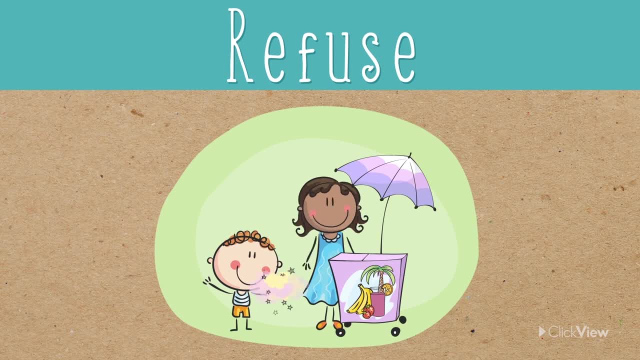 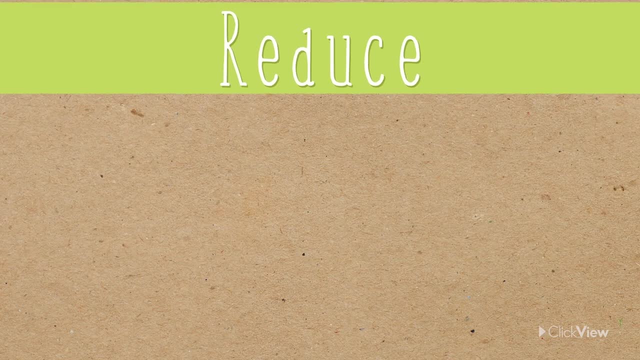 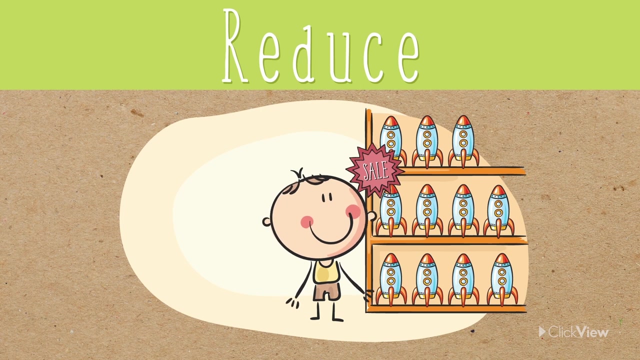 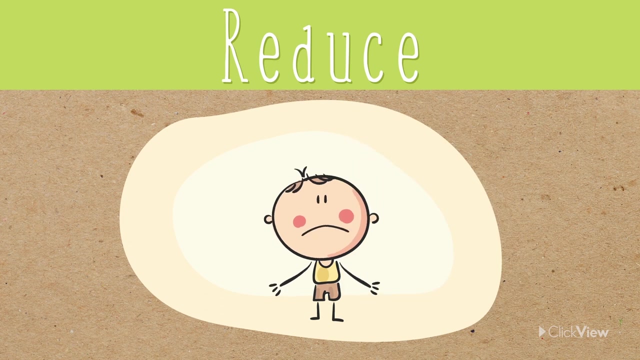 with a reusable straw Or, even better, no straw at all. Reduce means to use less. Sometimes it's hard to stop using resources completely, But you can always try to reduce the amount we use. You can save materials by buying fewer new toys. 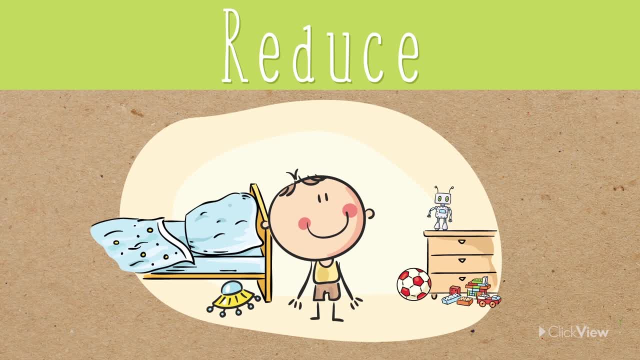 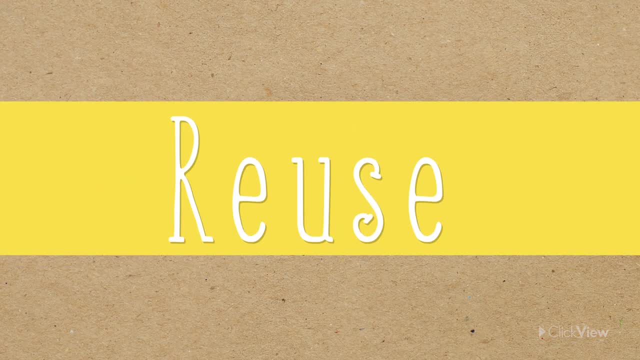 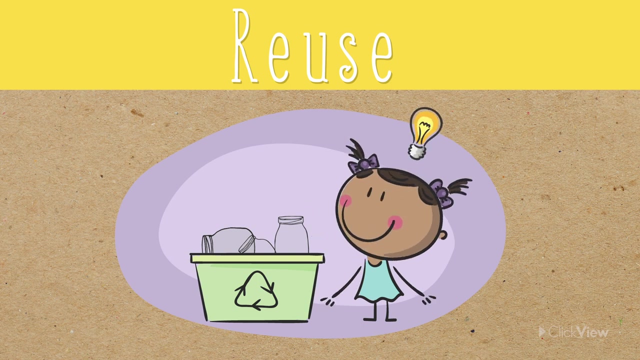 Before you get something new, have a look at what you already have. You might find you've got exactly what you need. Reuse means to use resources in a new way once we have finished using them for their original purpose. This is an opportunity to get creative. Instead of throwing an item out, think of another way you could use it. 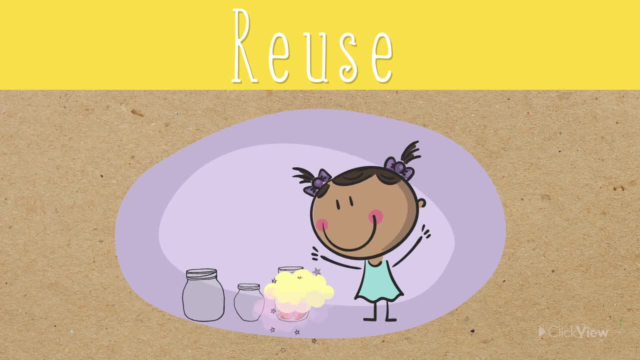 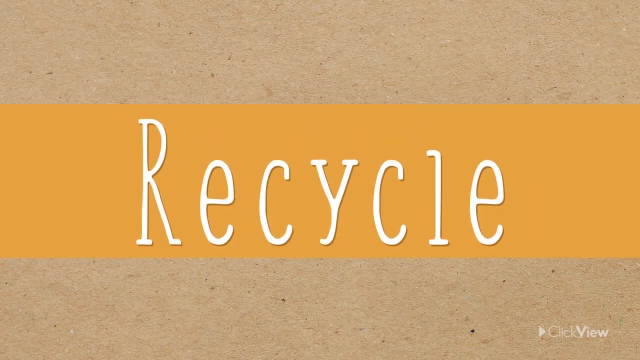 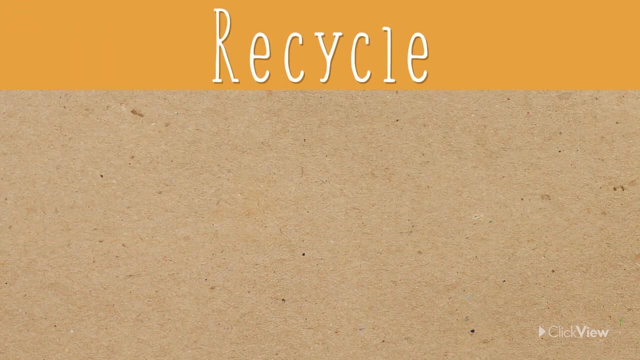 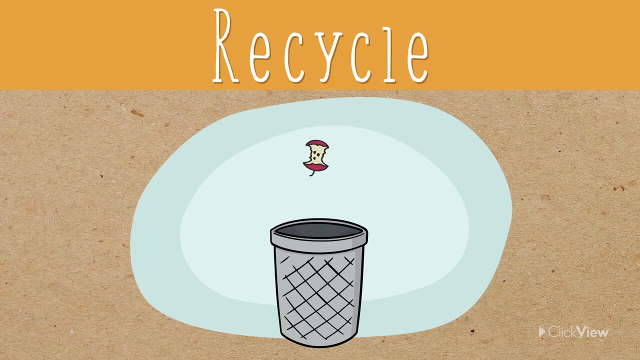 You could use empty jars as food containers, pencil holders or flowerpots. Recycle means to reuse. Recycle means to transform waste into things we can use again. When we throw something away, it's important to know what it's made of and how it should be thrown away.